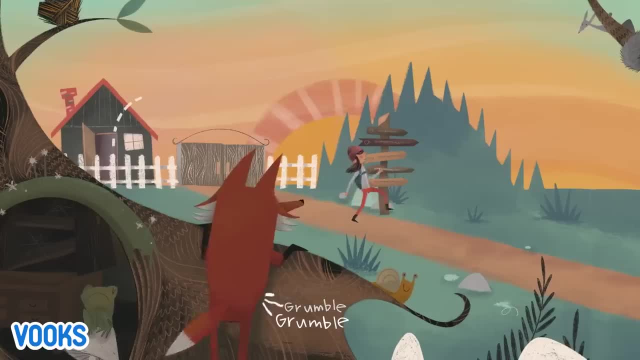 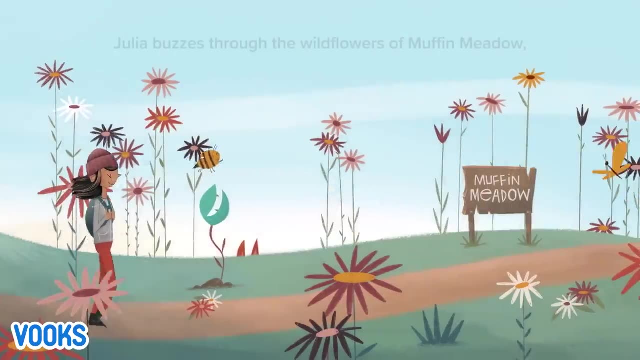 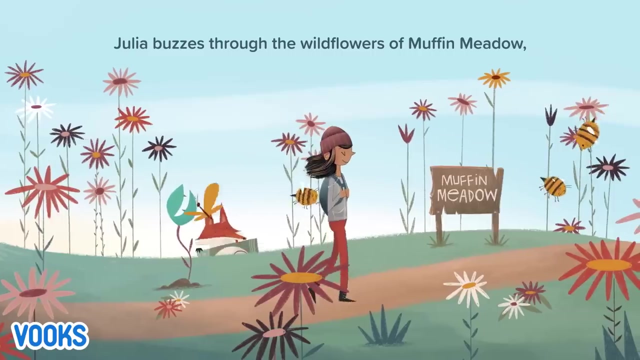 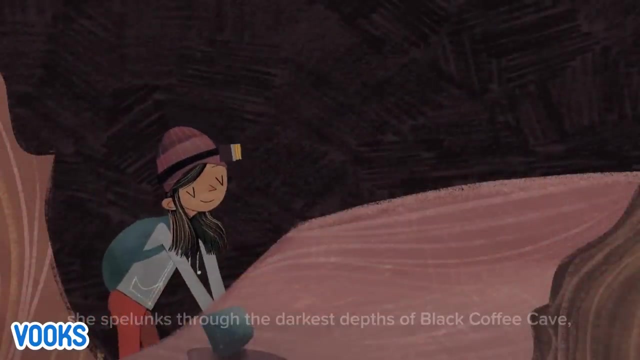 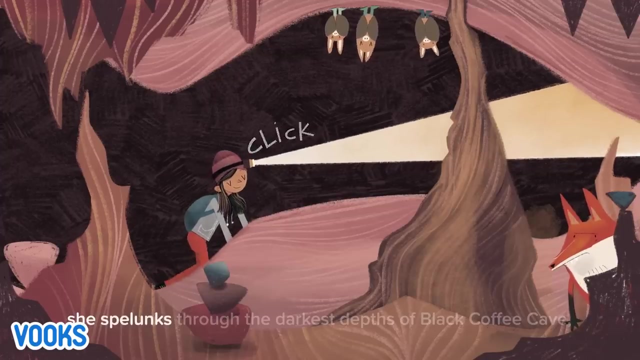 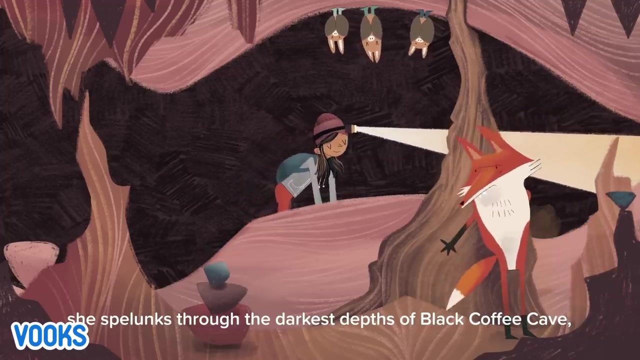 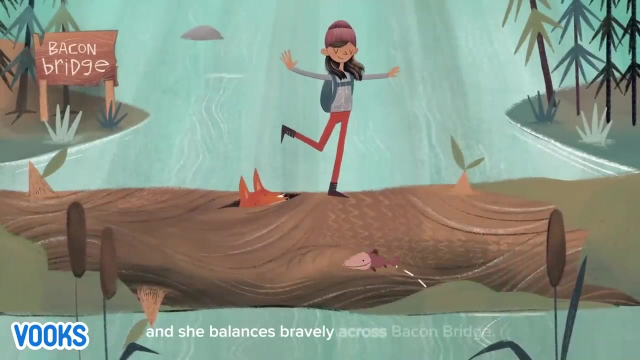 Grumble, grumble, grumble. Be home in time for dinner. Julia buzzes through the wildflowers of Muffin Meadow Click, She spelunks through the darkest depths of Black Coffee Cave And she balances bravely across Bacon Bridge. 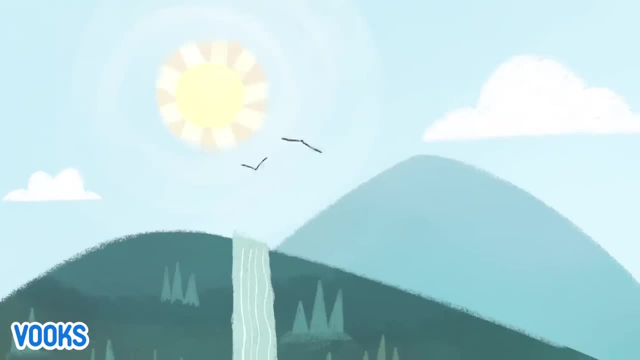 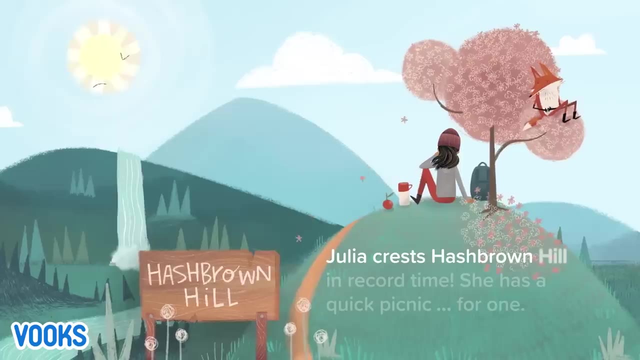 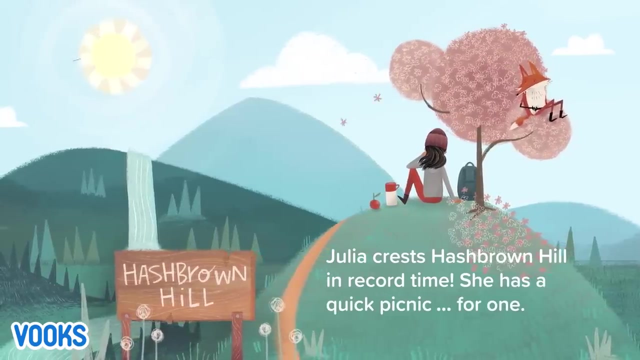 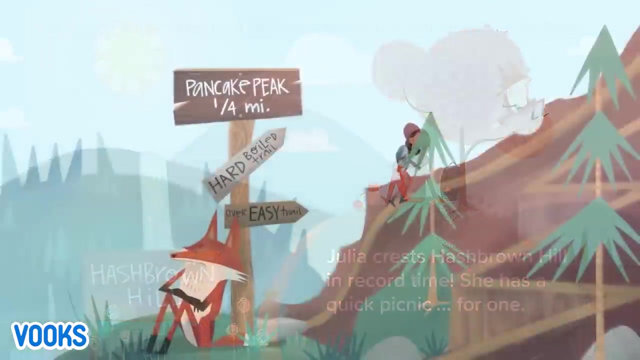 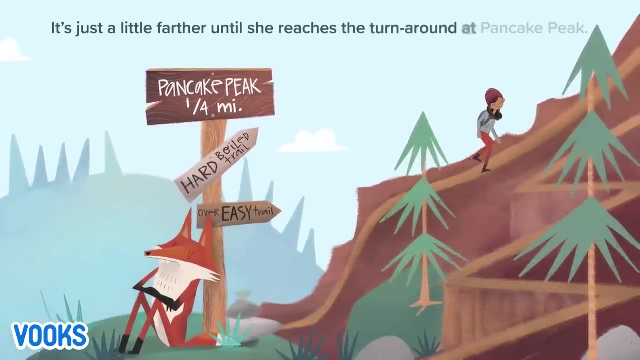 Julia crests, Hashbrown Hill. in record time She has a quick picnic for one. Grumble, grumble, grumble. It's just a little farther until she reaches the turnaround at Pancake Peak: Grumble, grumble, grumble. 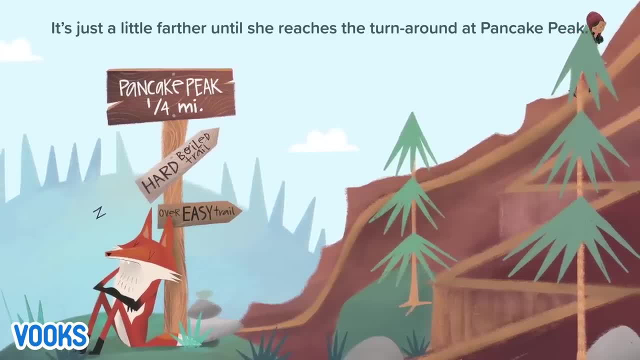 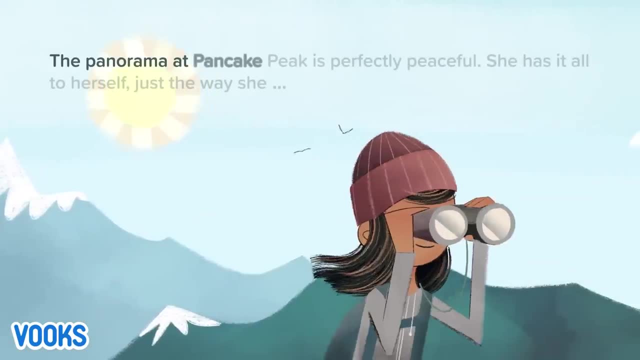 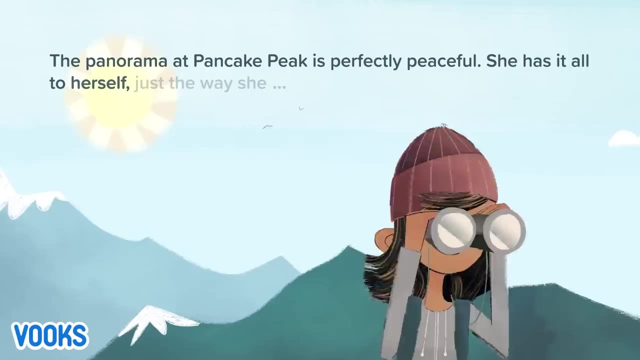 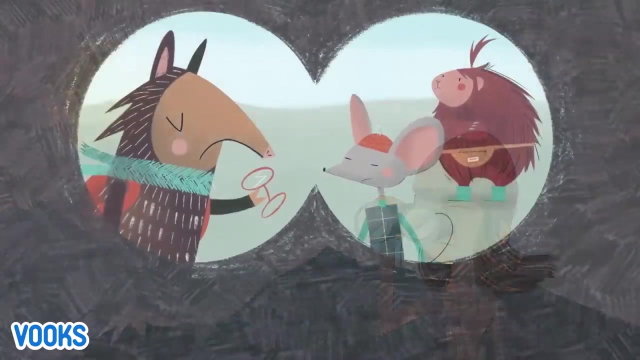 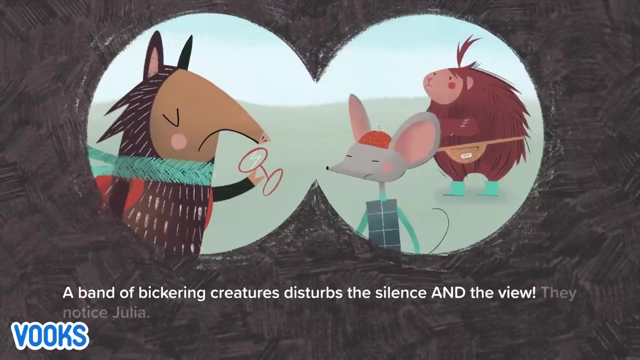 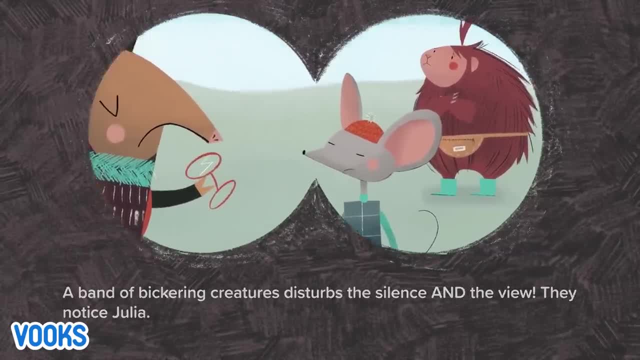 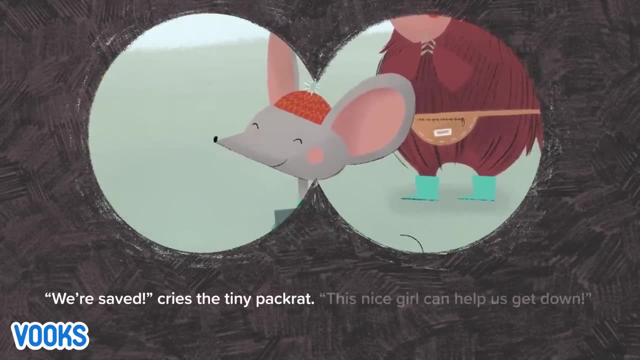 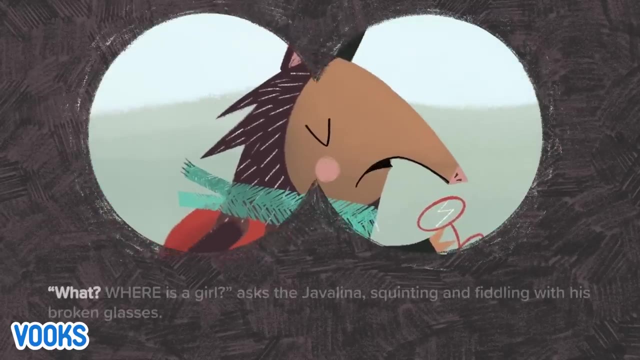 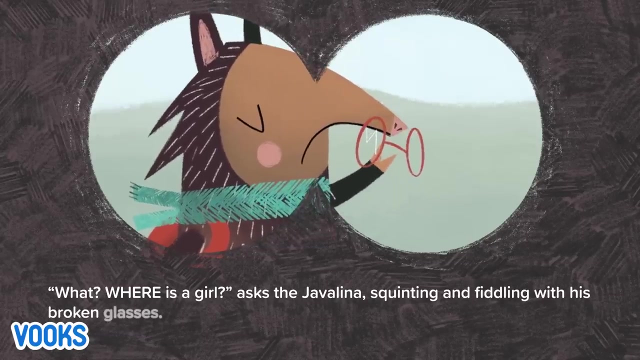 They notice. Julia, We're saved, Cries the tiny pack rat. This nice girl can help us get down. What? Where is a girl, Asks the javelina, squinting and fiddling with his broken glasses. A stranger. 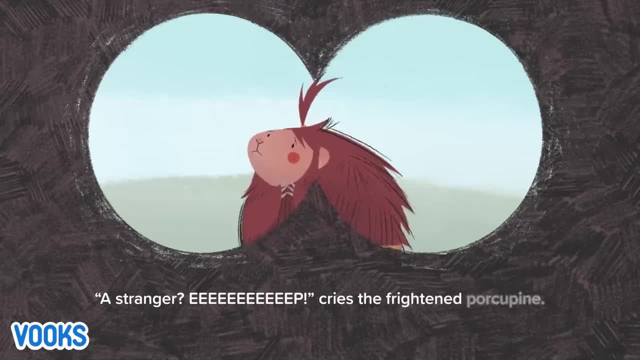 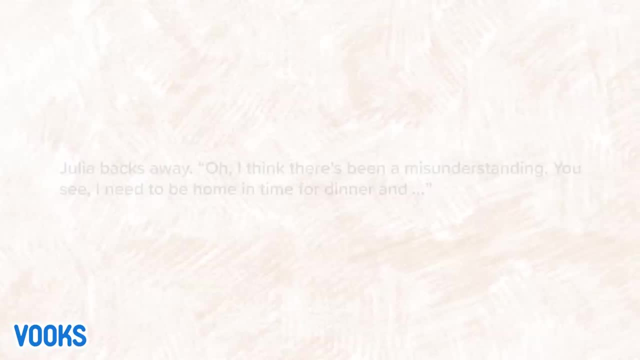 Eeeep, Cries the frightened porcupine. Julia backs away. Oh, I think there's been a misunderstanding. You see, I need to be home in time for dinner and My name's Fitz Interrupts the pack rat. 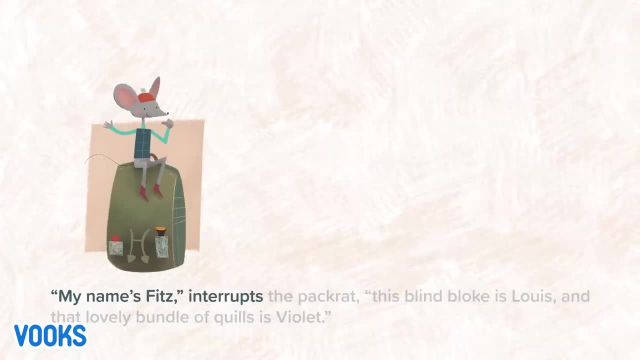 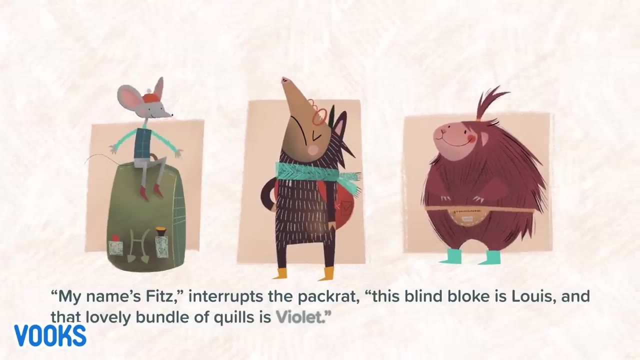 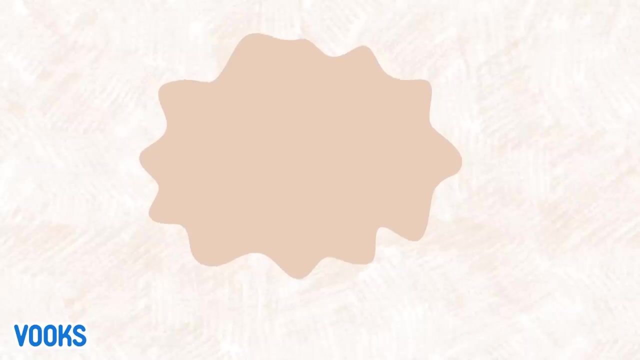 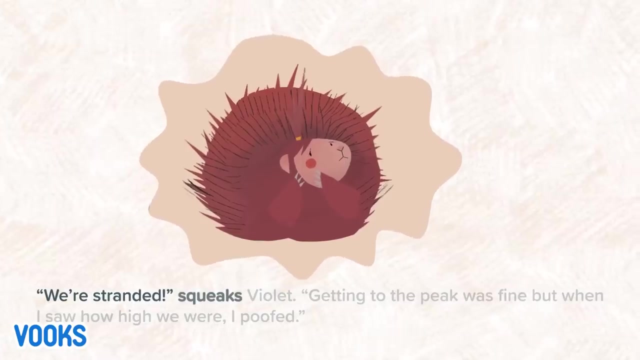 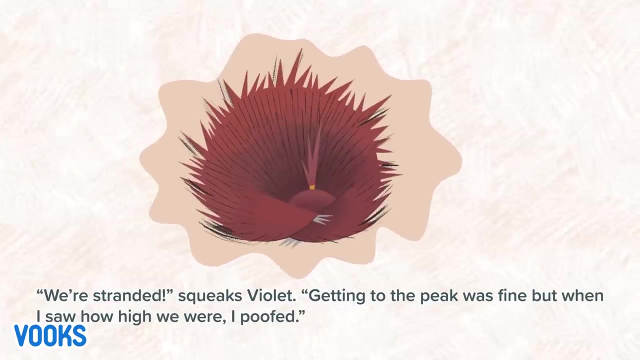 This blind bloke is Lewis and that lovely bundle of quills is Violet. Julia's back, This is Violet. We're stranded, Squeaks Violet. Getting to the peak was fine, but when I saw how high we were, I poofed. 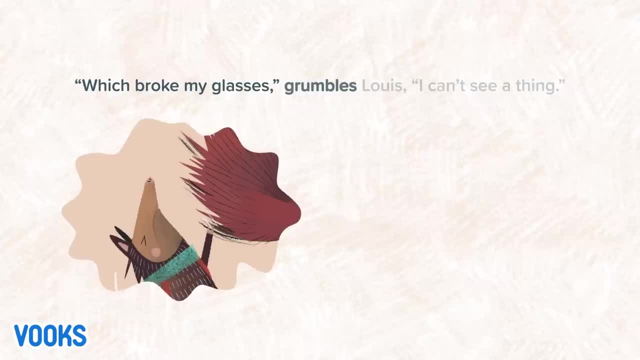 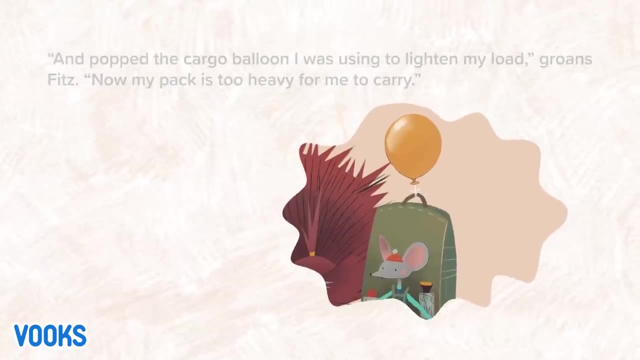 Which broke my glasses- Grumbles Lewis, I can't see a thing- And popped the cargo balloon I was using to lighten my load. Groans Fitz, Now my pack is too heavy for me to carry, So What do you say? 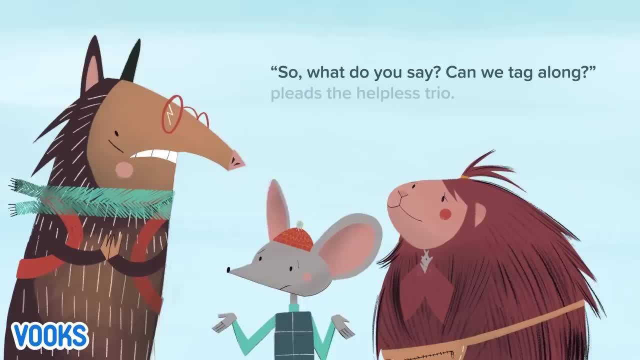 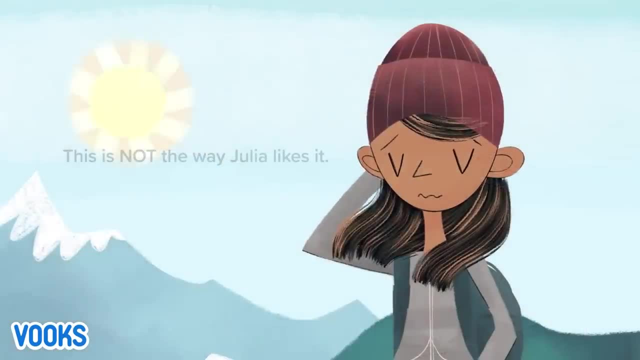 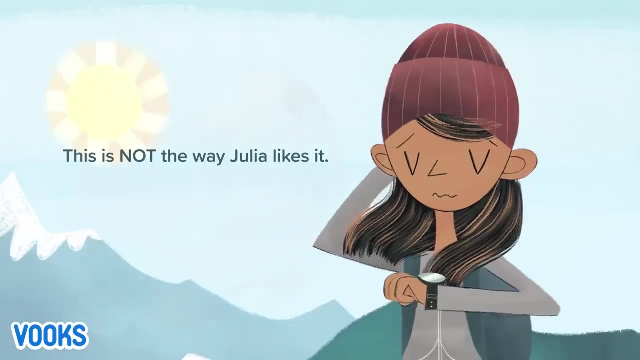 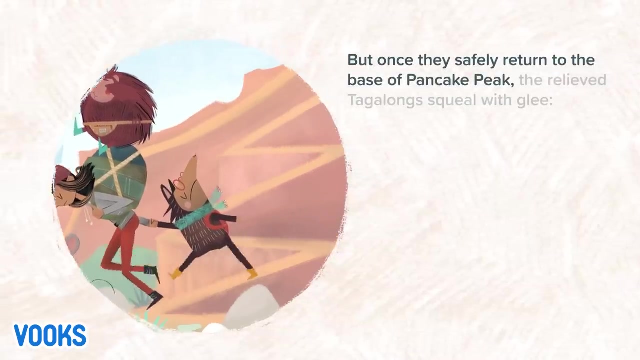 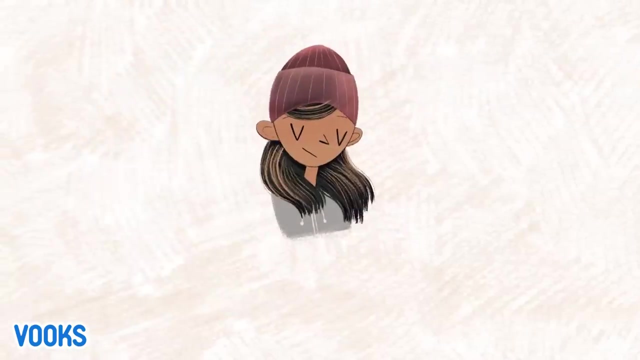 Can we go See? Can we tag along? Pleads the helpless trio. This is not the way Julia likes it, But once they safely return to the base of Pancake Peak, the relieved tagalongs squeal with glee. Julia, 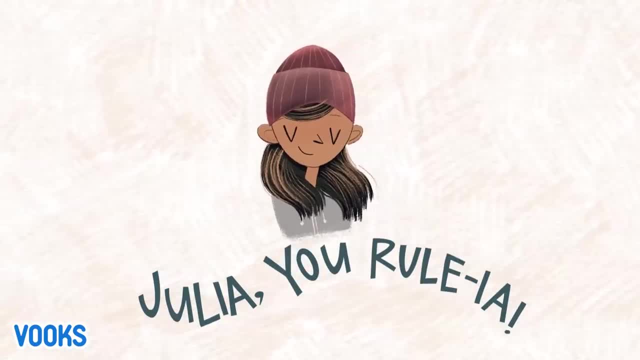 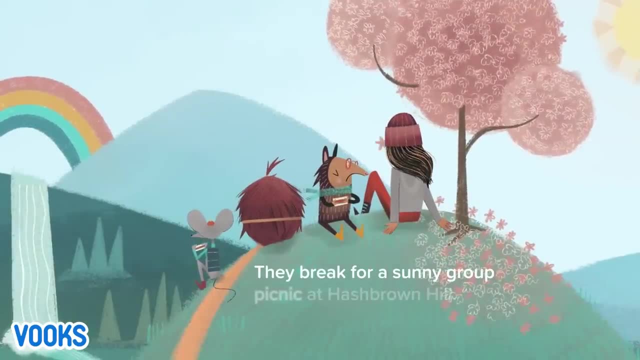 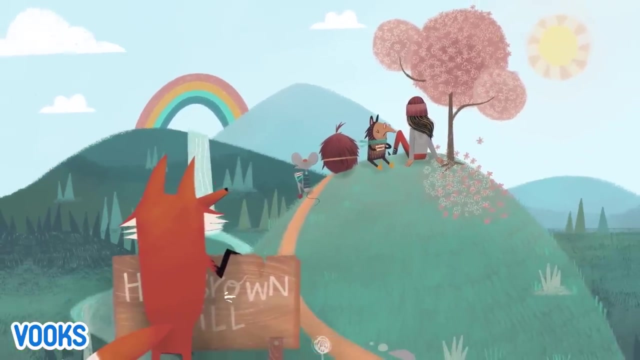 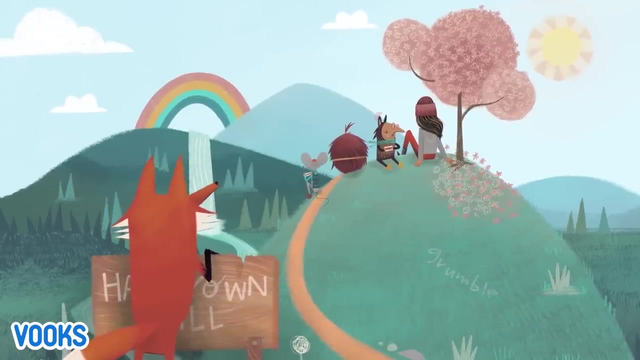 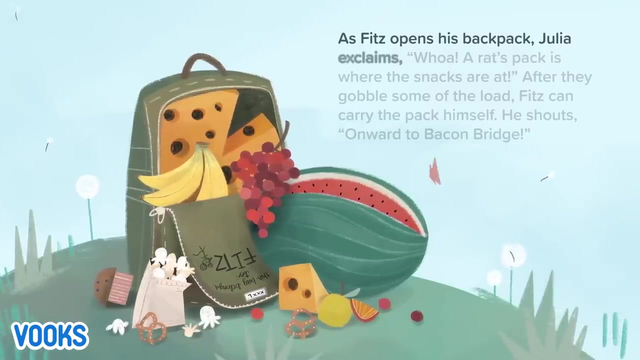 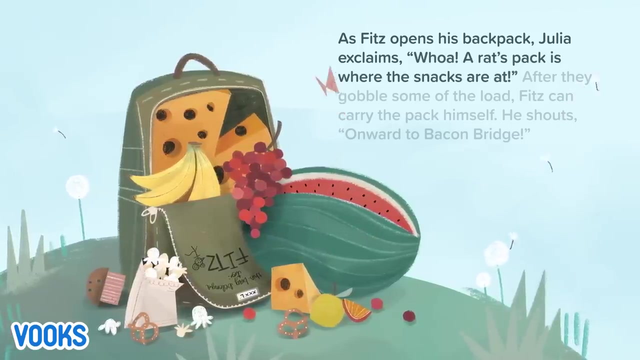 You, Rulia. They break for a sunny group picnic at Hashbrown Hill. Grumble, grumble, grumble. As Fitz opens his backpack, Julia exclaims: Whoa, A rat's pack is where the snacks are at After they gobble some of the load. 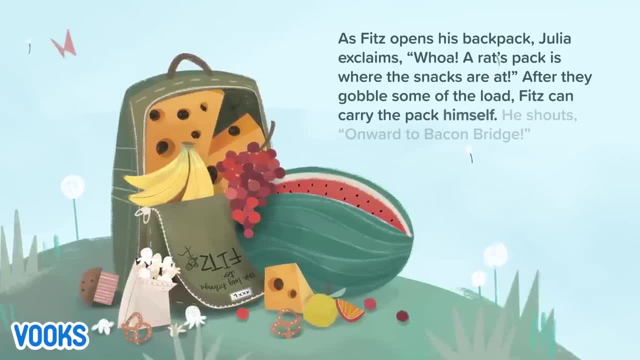 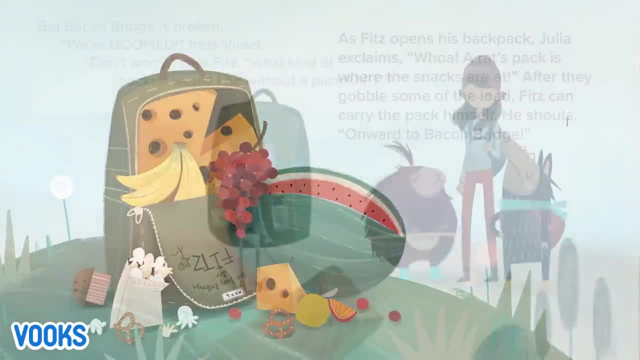 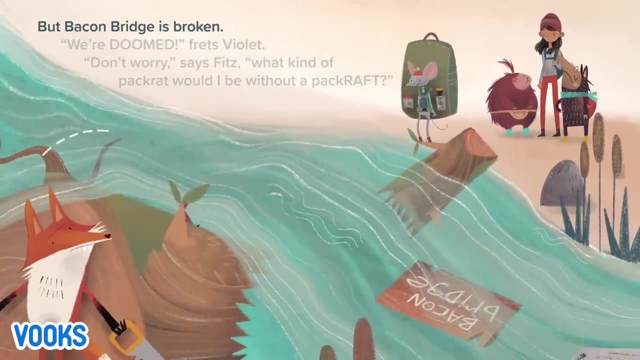 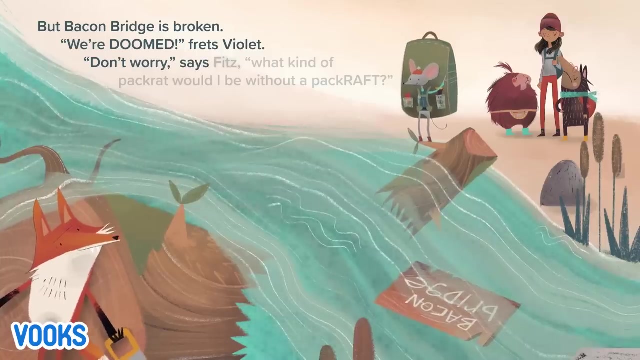 Fitz can carry the pack himself. He shouts Onward to Bacon Bridge. But Bacon Bridge is broken. We're doomed. Fretts, Violet, Don't worry, Says Fitz. What kind of pack rat would I be without a pack rat? 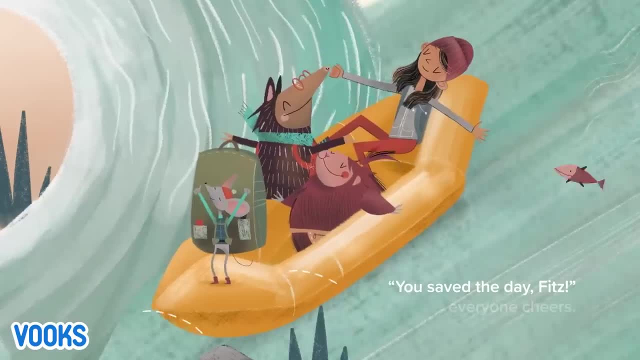 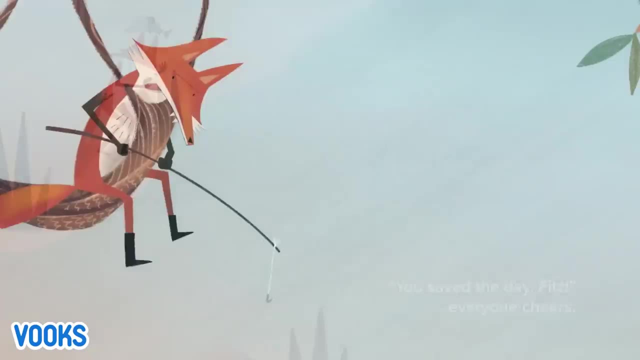 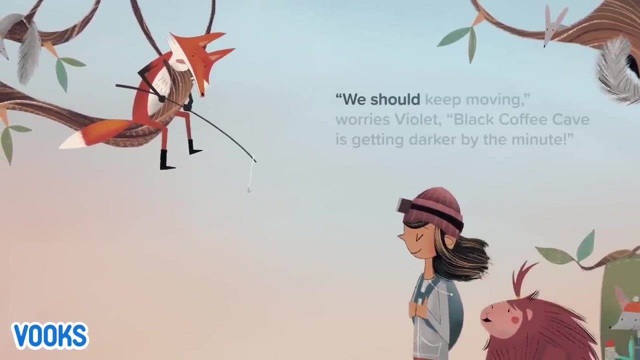 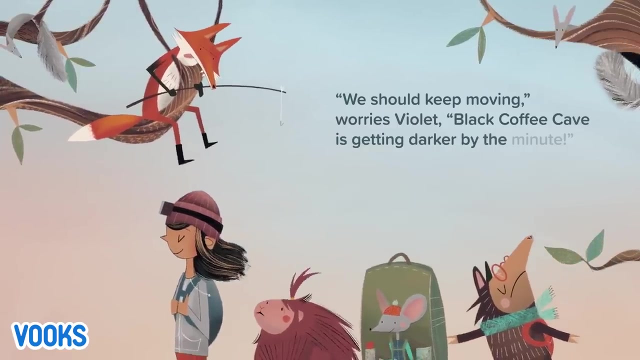 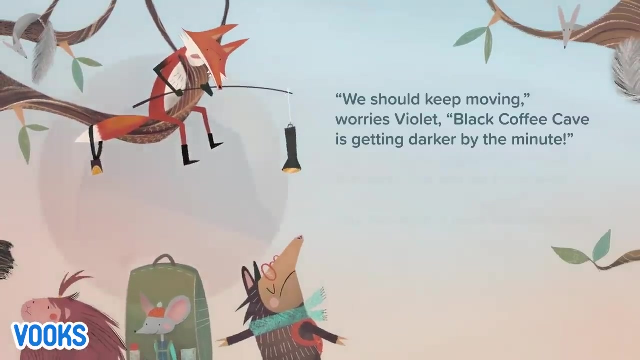 You saved the day, Fitz. Everyone cheers. We should keep moving Worries. Violet Black Coffee Cave is getting darker by the minute. Oh no, Julia gasps at the mouth of the cave. Oh no, We're stuck. 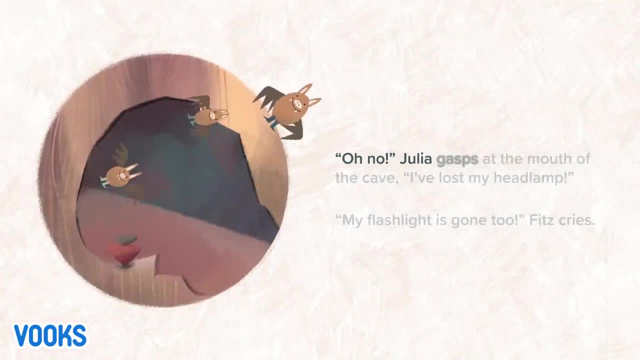 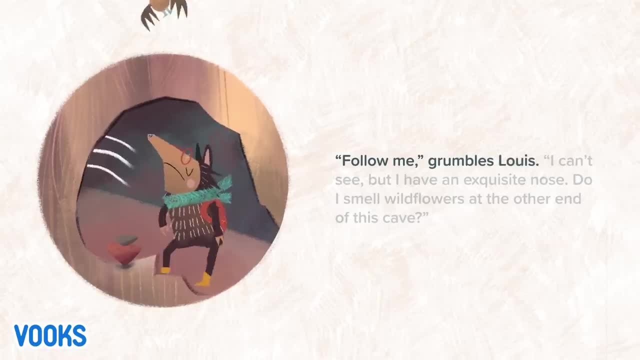 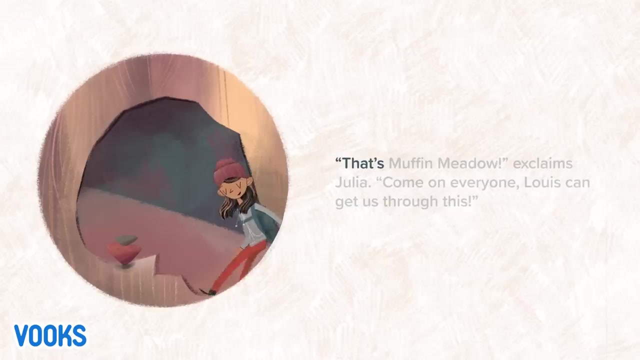 Do I smell wildflowers at the other end of this cave image? 그 It's all right, We can't stand out. Also, something smells rotten inside this Mason tree box. It could be some food. That's Muffin Meadow, exclaims Julia. 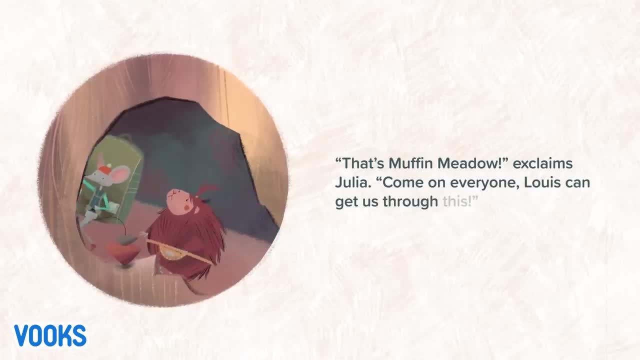 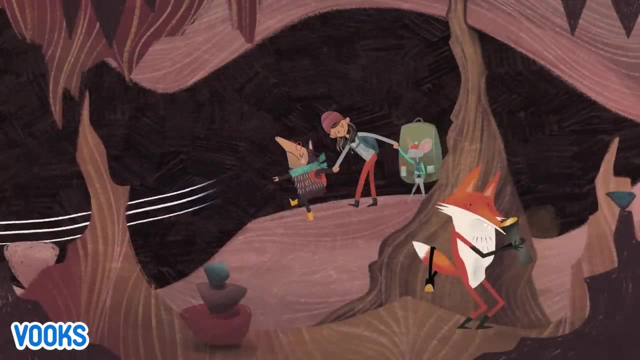 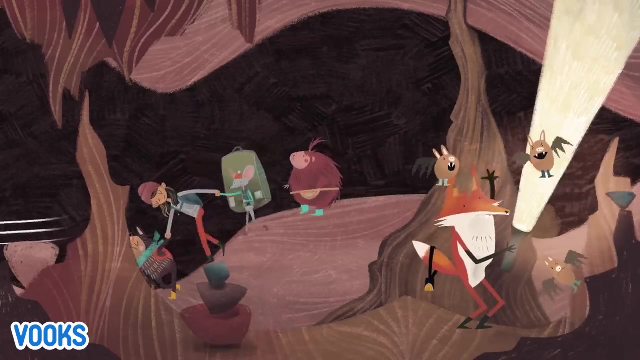 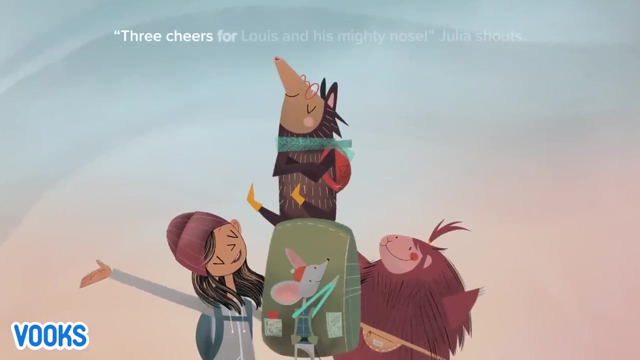 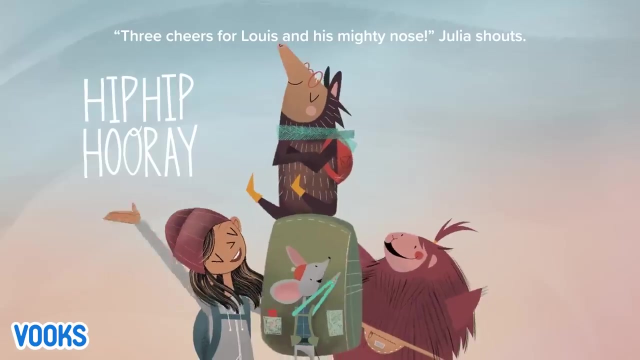 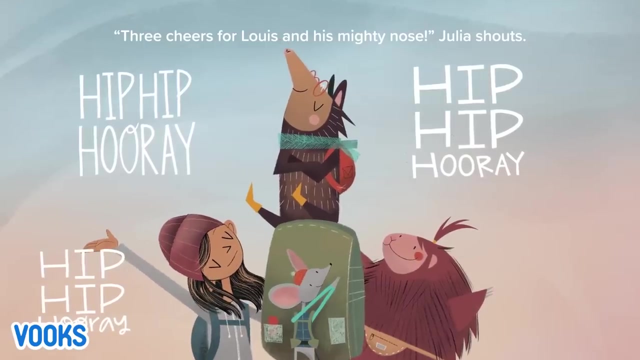 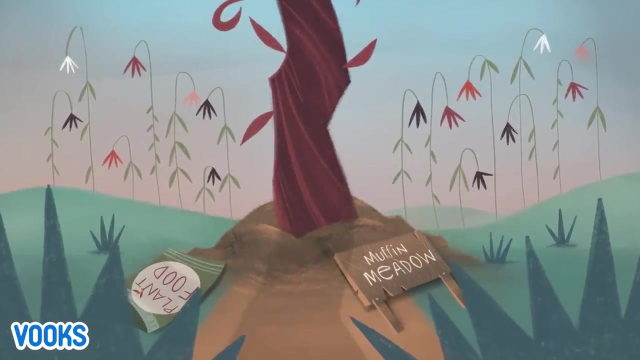 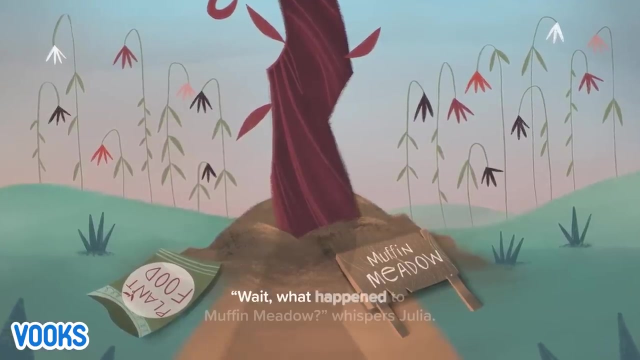 Come on everyone. Lewis can get us through this. Three cheers for Lewis and his mighty nose. Julia shouts Hip hip hooray, Hip, hip hooray, Hip, hip hooray. Wait, what happened to Muffin Meadow? whispers Julia. 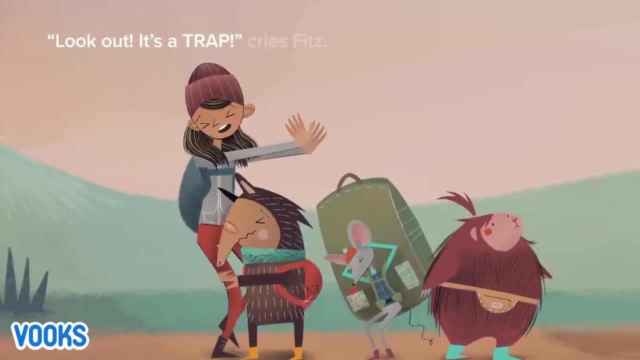 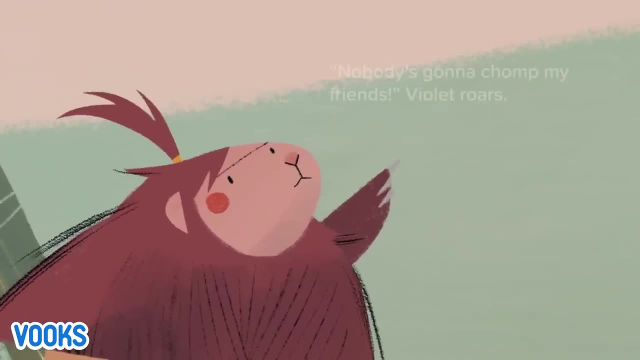 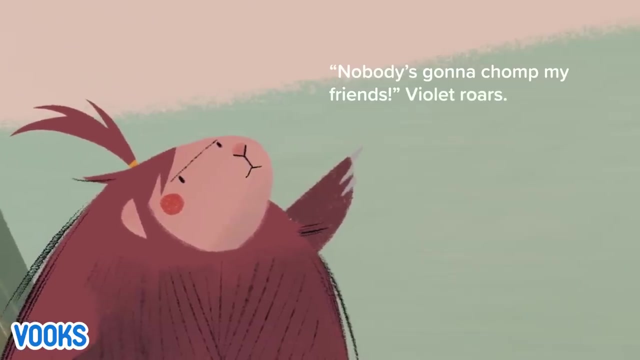 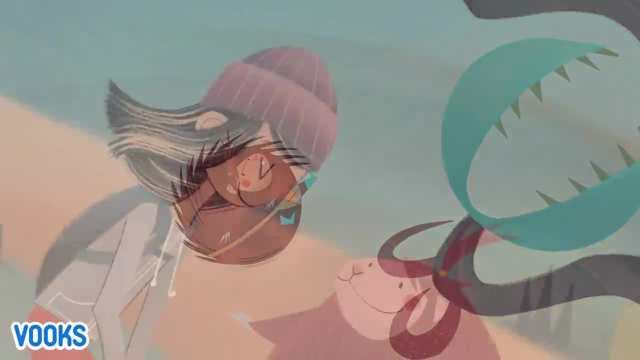 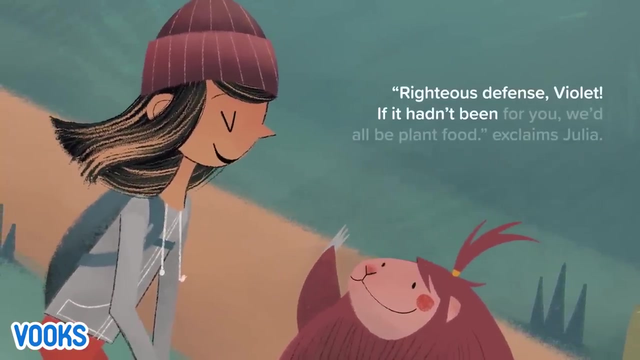 Look out, It's a trap, Cries Fitz. Nobody's gonna chomp my friends. Violet, roars, Eeeeee-choo. Righteous defense, Violet. If it hadn't been for you, we'd all be plant food. exclaims Julia.